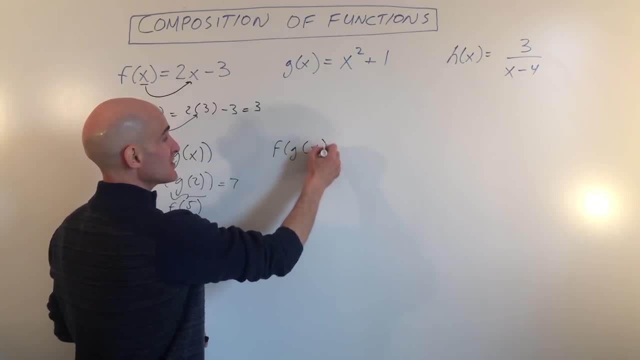 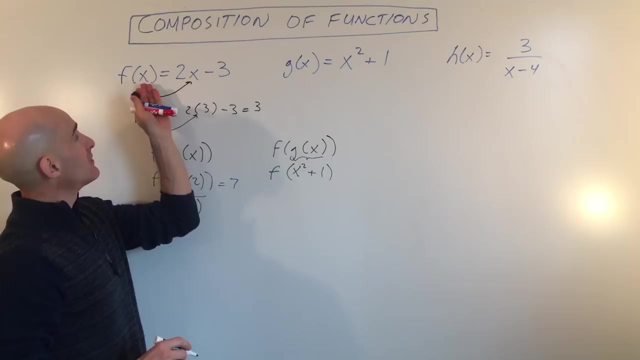 So we're going to just calculate what f of g of x is. Okay, so g of x is x squared plus 1.. So I'm going to substitute that in for g of x. okay, like? so, All right with me so far. So then, what we're going to do is we're going to put this quantity into our f function. 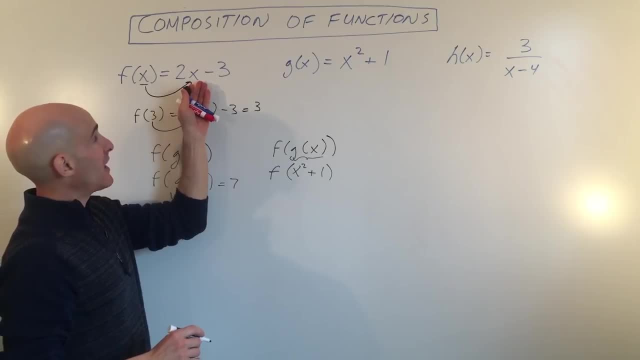 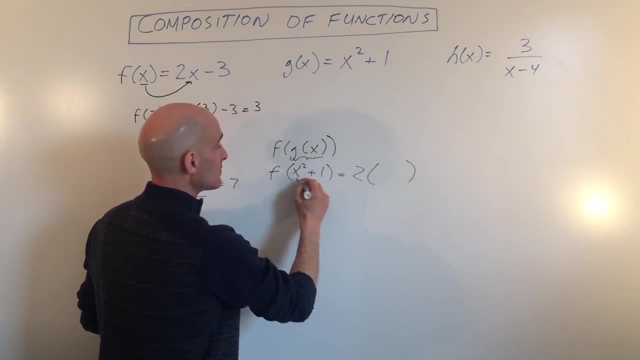 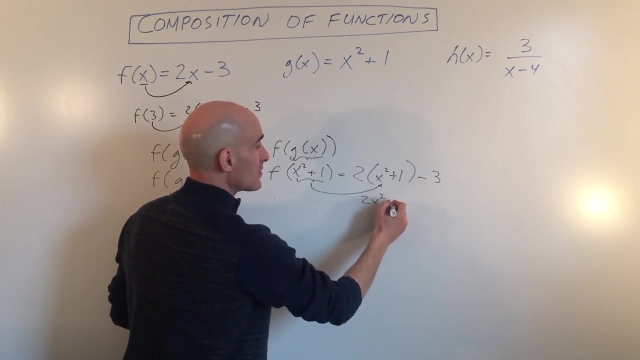 So remember whatever is in parentheses goes in place for x on the right side of the equation. So this is going to be equals 2 times- this is our input- x squared plus 1 minus 3.. So that comes out to 2x squared plus 2 minus 3, which is 2x squared minus 1.. 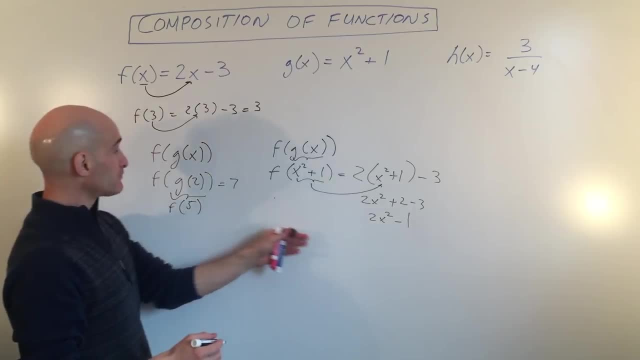 Okay, so this is what f of g of x equals: 2x squared minus 1.. If we were to go back to this previous example where we found out f of g of 2, what we can do now is we can put 2 in. 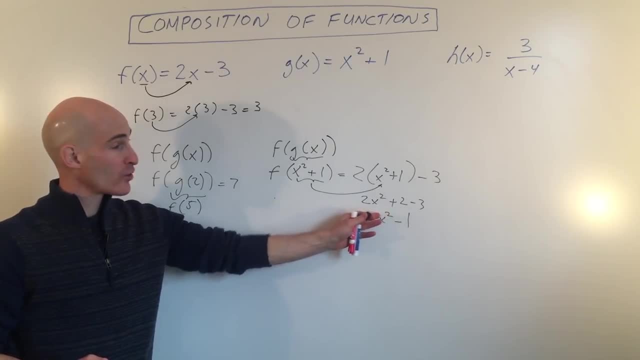 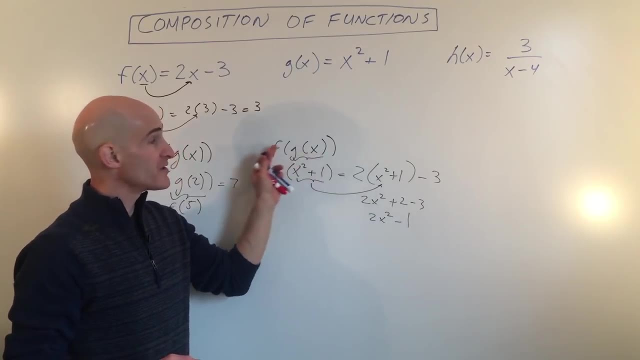 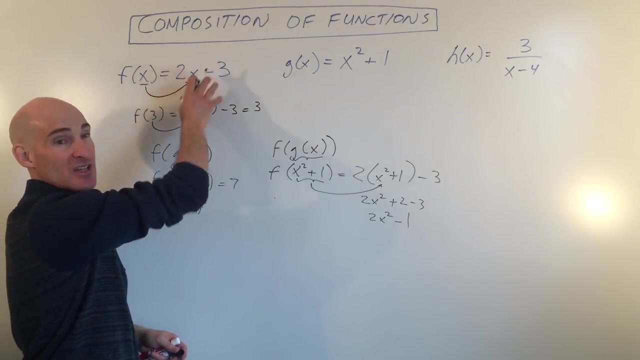 For x, 2 squared is 4 times 2, is 8 minus 1 is 7.. See, we have an expression now here that can do both of these operations all at once without having to go to the g function. find an answer. then put that into the f function: get an answer. 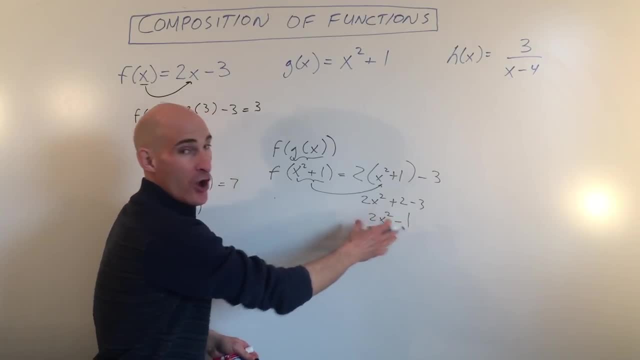 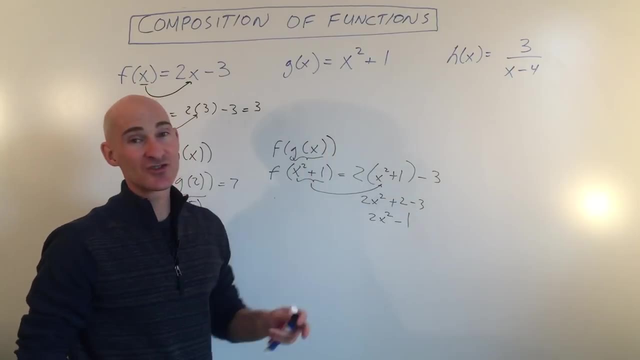 Here we have something that can do that operation all in one step. Okay, you just have to substitute into x and you're going to get the composition of these two functions together. Now, not to be confused here, if we were to write this as g of f of x, this is a completely different operation. 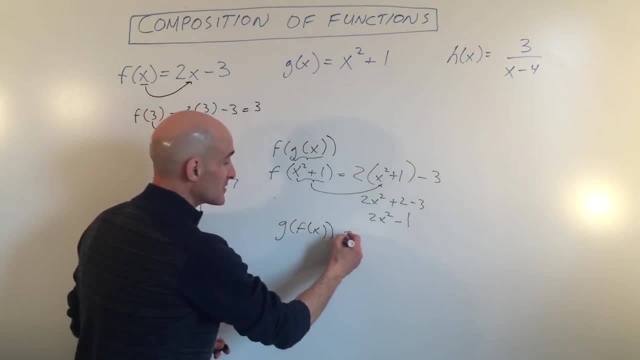 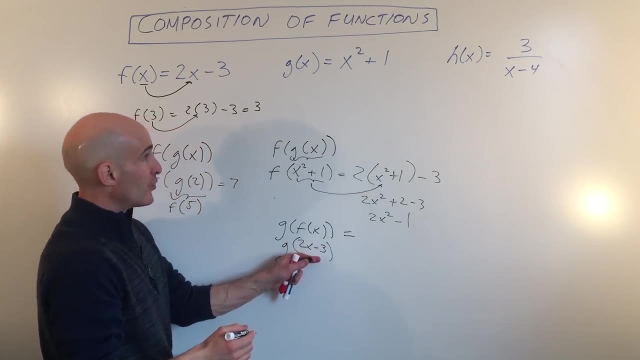 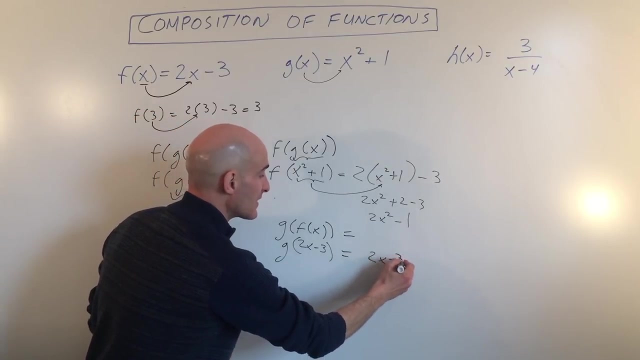 Here we're putting the f function into the g function. The way this would look is 2x minus 3, that's this quantity here. That's our input for our g function, So that's going to be- we're putting this in place of x, so that's going to be 2x minus 3.. 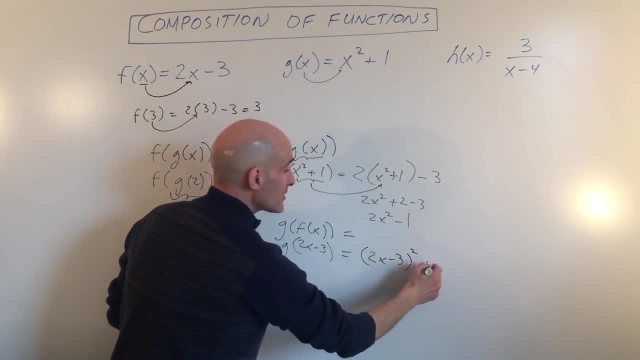 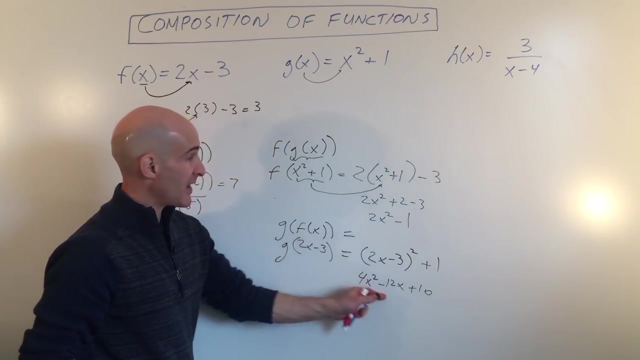 The quantity squared, because we're squaring our input plus 1.. If we simplify, we get 4x squared minus 12x, plus 9, plus 1 more, which is plus 10.. So here's f of this is g of f of x, which you can see is not the same as f of g of x. 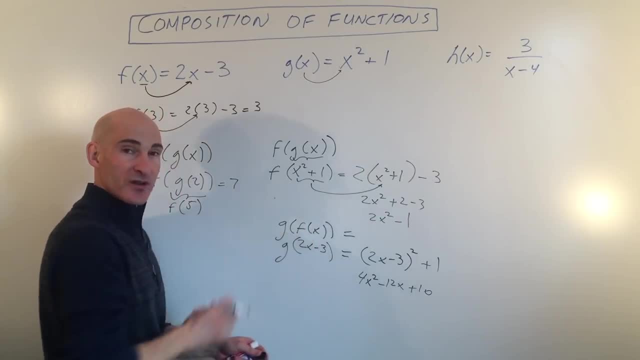 Okay. so the order is important, which one you're putting in first and which one second. So here's a couple examples- f of x, g of x, Composing the functions. I'm going to show you one last example here. 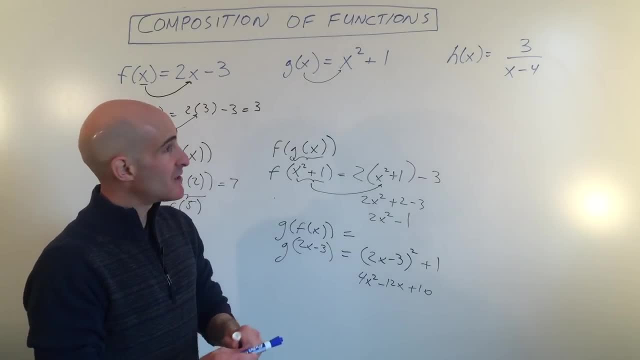 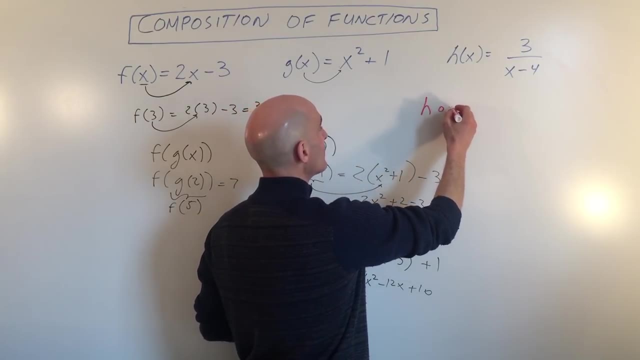 We've got another function, h of x. But I'm going to show you another notation that some books use, and that's this notation right here. Say, you had h of f, Okay, so you see this notation here. This is the same thing as h of f of x. 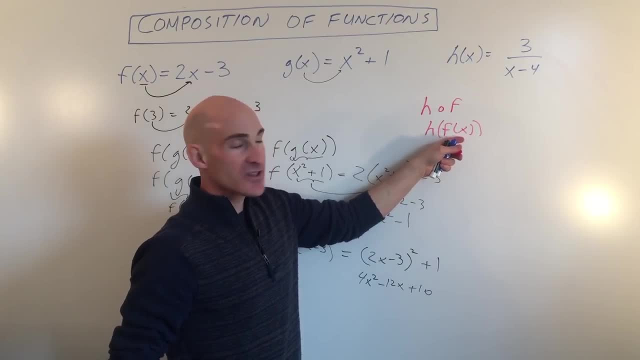 I prefer this notation because it looks like this is the inner print, So you're going to have parentheses and you're working from the inside out, like following your order of operations. Here it actually appears as if you're working from the right to the left, which is a little bit counterintuitive for some students. 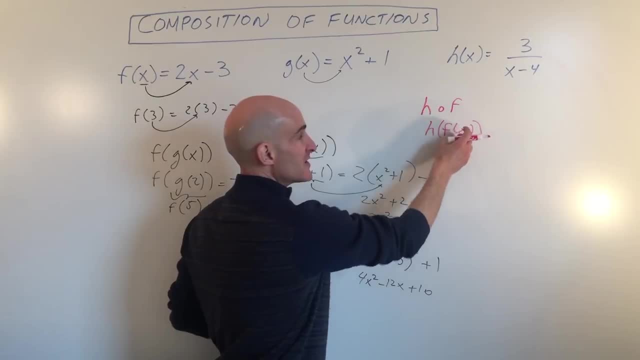 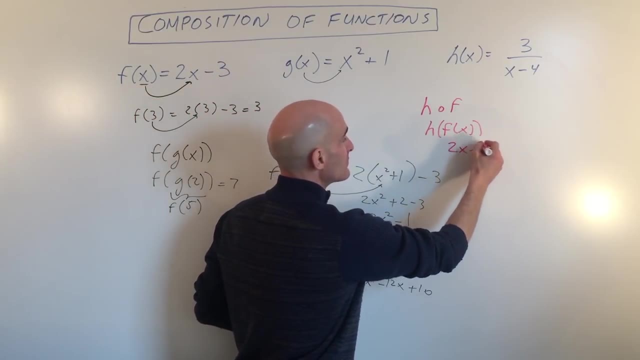 because we're used to reading from left to right, But what you're actually doing is you're working from the inside out. So to find this, h of f of x, f of x is 2x minus 3, 2x minus 3.. 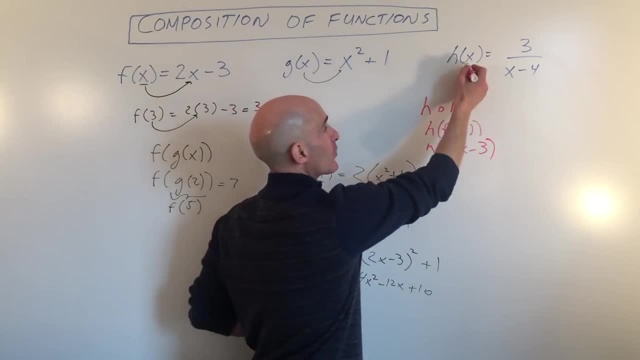 And we're putting that into our h function. Okay, so for whatever's in parentheses here, that's our input. That's going in for x on the right side. Okay, So this is going in for x on the right side. 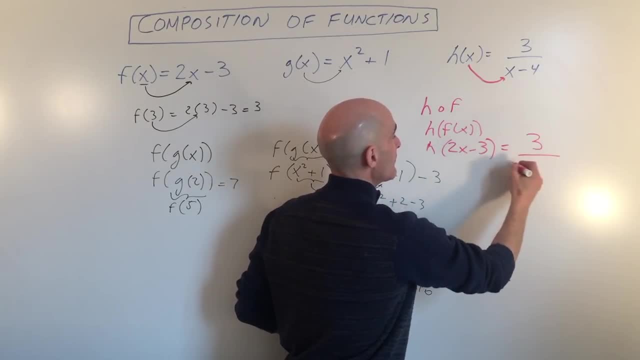 So this is going in for x on the left side. So this is going in for x on the right side. So this is going in for x on the right side. So this is going to equal 3 divided by 2x minus 3 minus 4.. 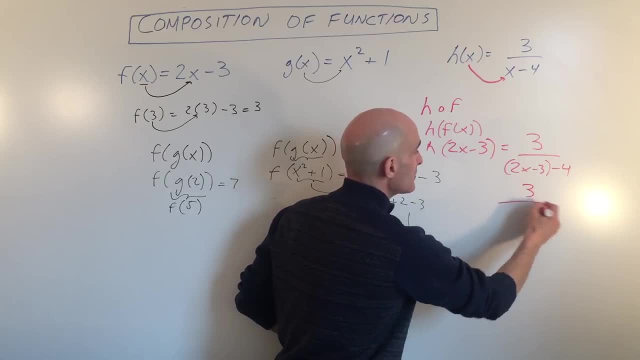 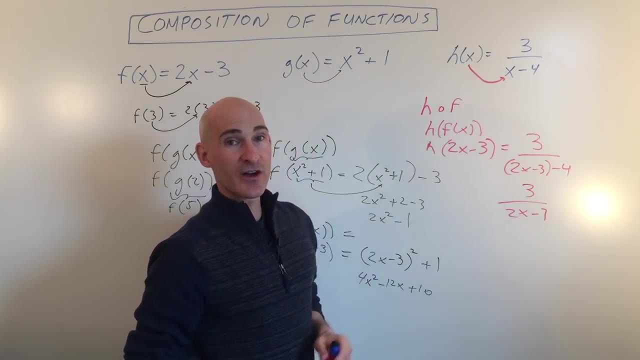 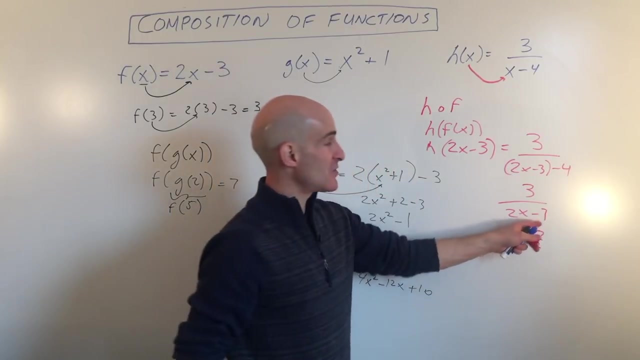 And you can simplify that down a little bit further. That's going to be 3 divided by 2x minus 7.. And so there you go. That's a composition of functions. One thing you want to notice here is that x cannot equal 7 halves, because then you'd be dividing by 0.. 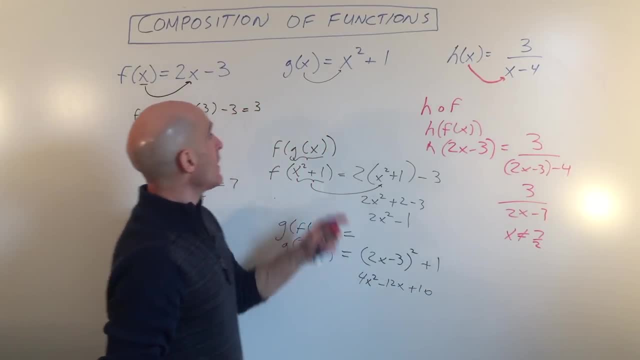 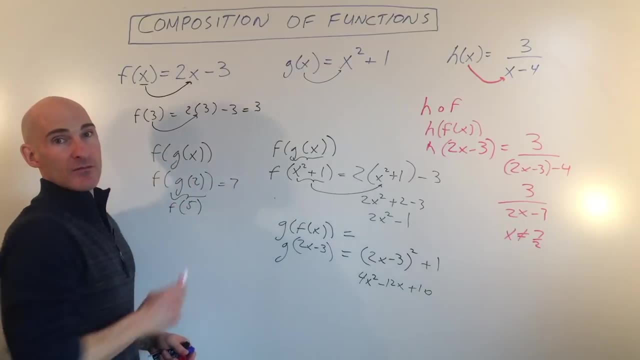 So that's a restriction on the domain, Something you want to watch out for. But go ahead and review this video. Composition of Functions. If you have a value, you can just go ahead and do it in multiple steps. But if you want to just find like a generic formula for the composition of the two functions, these are the steps that you're going to want to go through, So I'll see you in the next video.